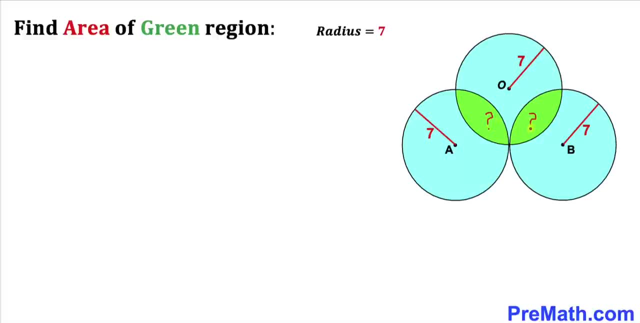 the area of this green shaded region. Please don't forget to give a thumbs up and subscribe. Let me make it very clear that this figure may not be 100% true to the scale. Let's go ahead and get started with the solution, and here's the very first step. Let's make an observation. 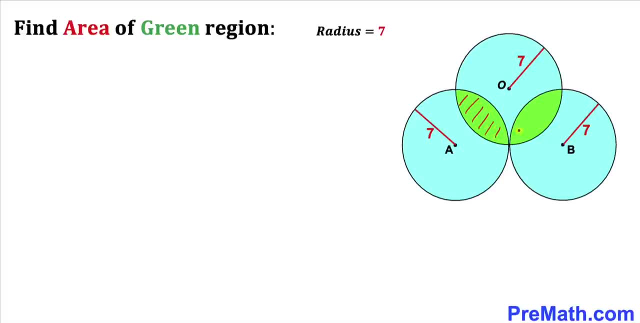 since we are going to calculate the area of this green shaded region. So therefore, we are going to focus on this semi-circle and we can see that this green region area is equal to the area of this whole semi-circle minus the area of this brown shaded region, as you can see in this equation, and now we can easily. 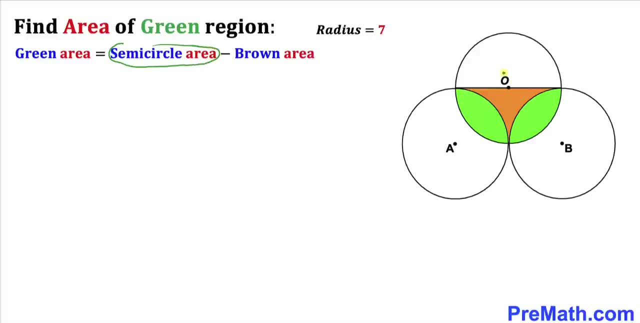 calculate the area of this semi-circle, since we know the radius is seven. and now let's recall the area of a circle. formula: area equals to pi r square. in our case, radius r is seven, so therefore the area of this semi-circle is seven, and now we can easily calculate the area of this semi-circle. 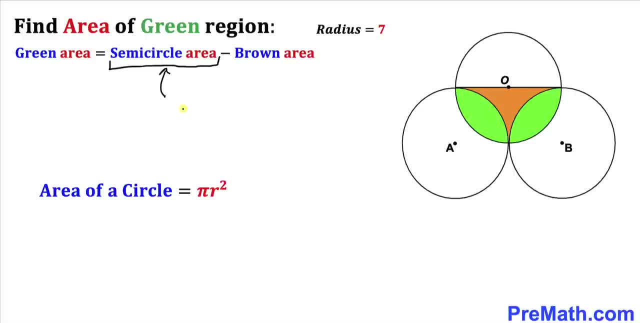 This is simply going to be pi. r, in our case, is seven whole square. since we are dealing with the semi-circle, we are going to divide it by two. so therefore, if we simplify this thing, that is going to give us 49 pi divided by two, and that is going to be the area of this semi-circle. so therefore, 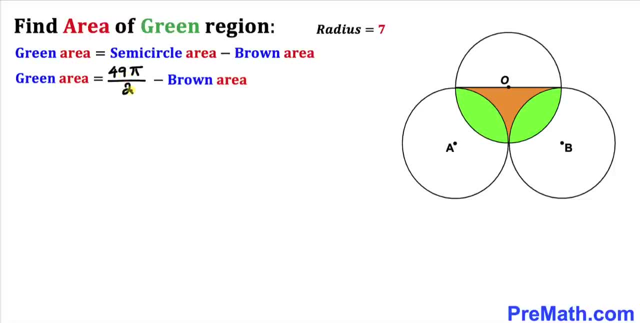 the green shaded area turns out to be 49 pi divided by two, minus this brown area. Let's go ahead and call this our equation number one. and now our task is to calculate the area of this brown shaded, this region. and here's our next step. we got this rectangle a, b, c, d by connecting the 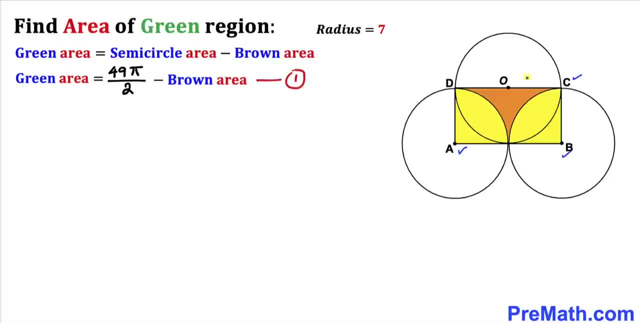 centers a, b, with these points c and d, as you can see in this diagram, and now we can see that this brown shaded area is equal to the area of this semi-circle. We got our rectangle that is equal to this area of this rectangle: a, b, c, d, minus the area of these two. 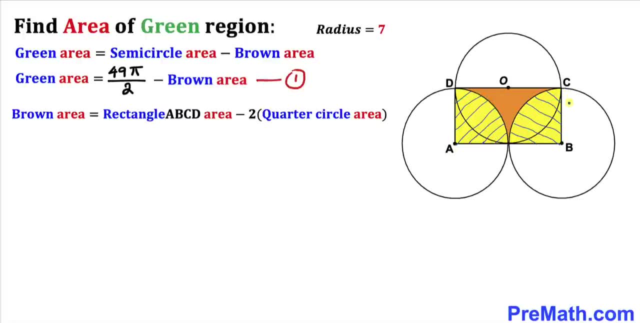 quarter circles, and now we know that the radius of this circle is seven units. so this side is going to be seven units and this is seven units. likewise, this side is seven units, since this radius, and this is seven units as well. So therefore, this distance a. 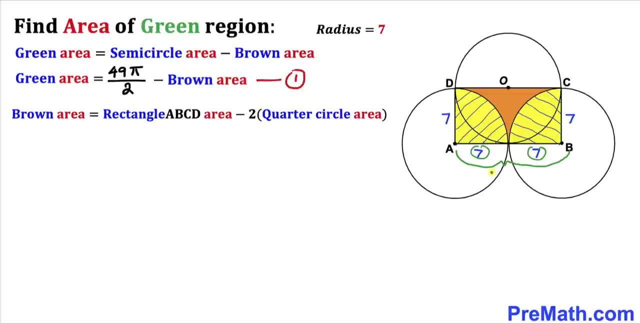 b is going to be 7 plus 7 is going to make 14 units. and here's our next step. let's go ahead and calculate the area of this rectangle: a, b, c, d. and now let's recall the area of rectangle. formula: area equals to length times width. in our case, the length of this rectangle is 14 and the width is 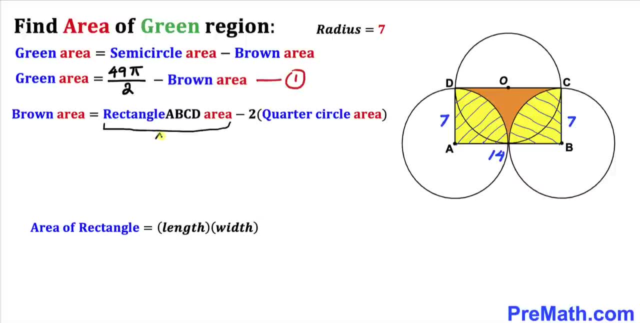 7 units. so therefore, the area for this rectangle a, b, c, d is going to be: in our case, length is 14 times width is 7, so that is going to give us 98 square units. so therefore, the area of this rectangle a, b, c, d turns out to be 98. and here's our next step. let's go ahead and calculate the. 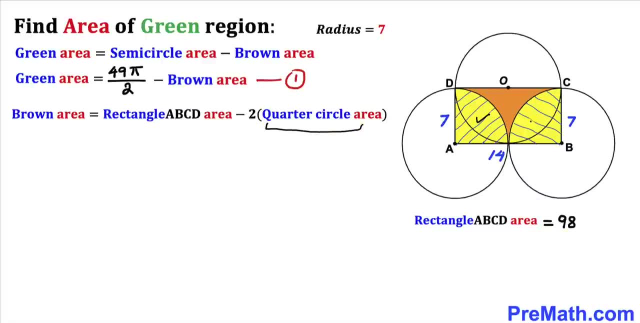 area of these quarter circles. now, and let's recall once again, the area of a circle, formula area equals to pi r square. so therefore the area of this quarter circle is going to be pi. radius, in our case is 7 whole square divided by. since we are dealing with this quarter circle, so we are going to divide by 4. let's simplify so. 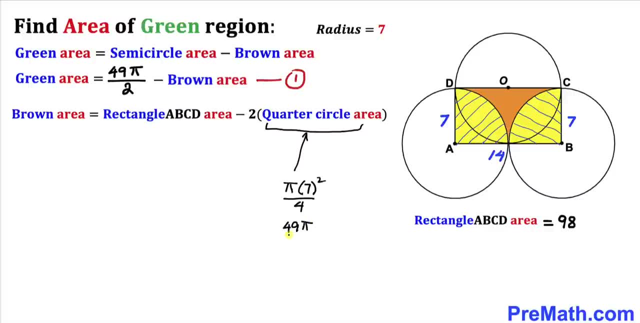 that is going to give us 49 pi divided by 4. now we can see. we got these two of these quarter circles, so i'm going to multiply this by 2, so therefore this quantity turns out to be 49 pi divided by 2. so therefore we can see the area of. 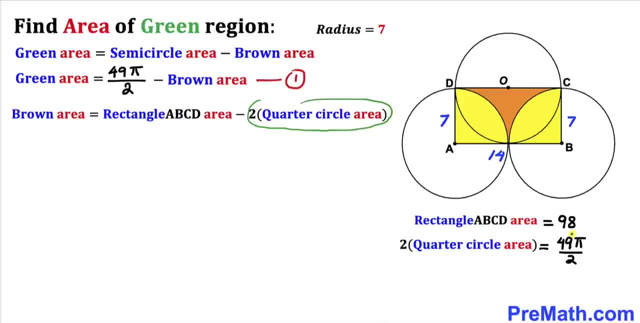 these two quarter circles turns out to be 49 pi divided by 2. and now we can easily calculate this brown area, since we already figured out our rectangle a, b, c, d area and the area of these two quarter circles. so therefore we are going to fill in the blanks. so this brown area is going to be equal to 98 minus 49 pi divided by 2. let me go. 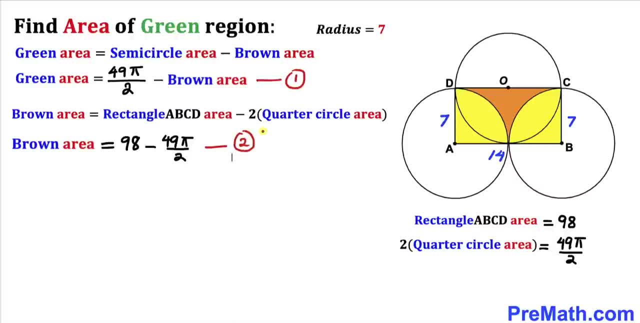 ahead and call this our equation number 2. and here's our final step. let's focus on our this equation 1 and we can see the green area is 49 pi divided by 2, minus this brown area, and we already figured out this brown area in this equation 2. and here's our equation 1, and let's go ahead and substitute this: 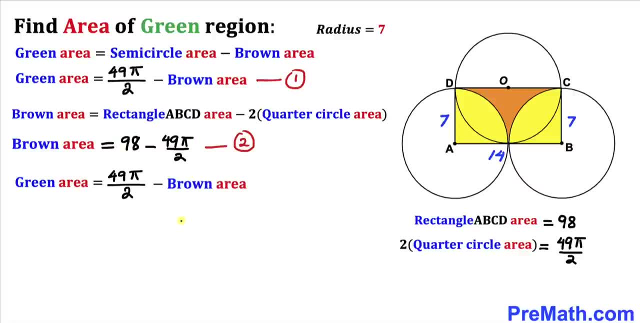 brown area value over here. so let's go ahead and substitute. so let me go ahead and copy down this part. first, 49 pi divided by 2, minus this brown area. I'm going to just copy down this one. so let me put a bracket over here: 98 minus 49 pi divided by 2. and now let's go ahead and distribute this. 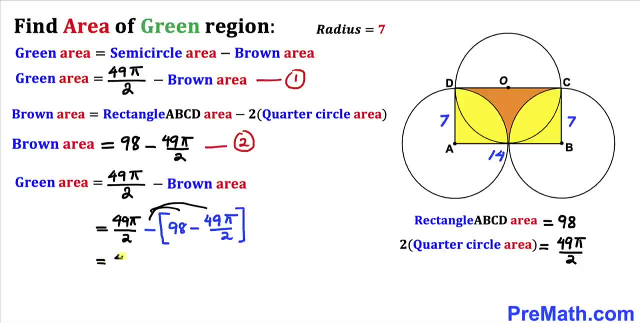 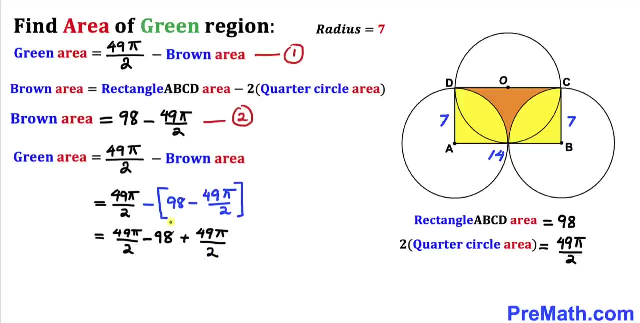 negative sign. so that is going to give us 49 pi divided by 2 minus 98. this negative and negative become positive: 49 pi divided by 2. and now let's go ahead and combine these like terms: 49 pi divided by 2 and this 49 pi divided by 2, and if we add these two numbers, that is going to give us simply: 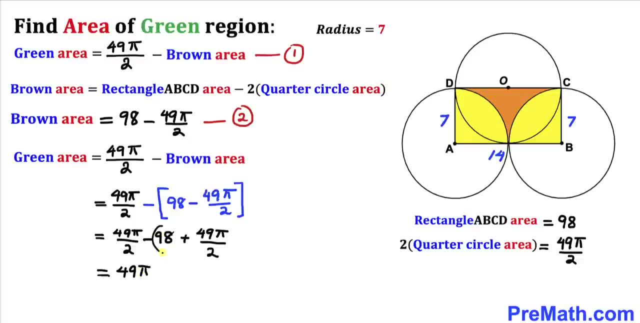 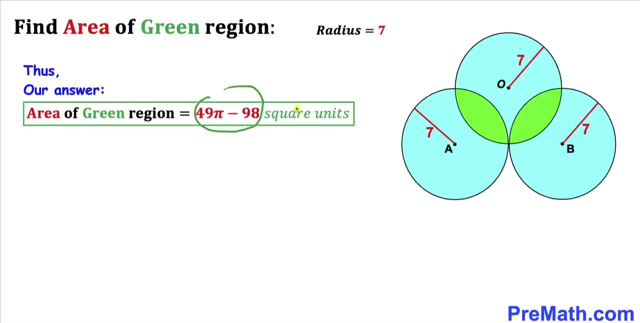 49 pi, and then I'm going to write down this- minus 98. so therefore, the green area turns out to be 49 pi minus 98. so thus the area of this green shaded region turns out to be 49 pi minus 98 square units, and that is approximately equal to 55.94 square units. thanks for watching and 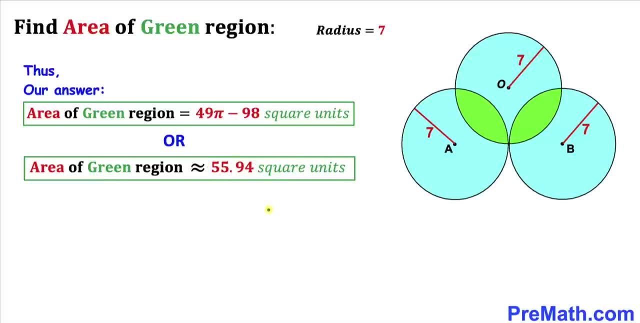 please don't forget to subscribe to my channel for more exciting videos. bye you.